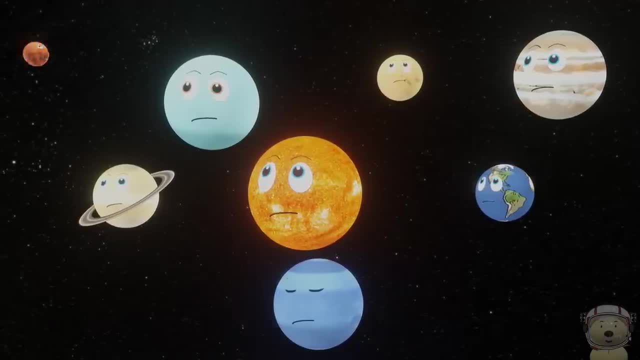 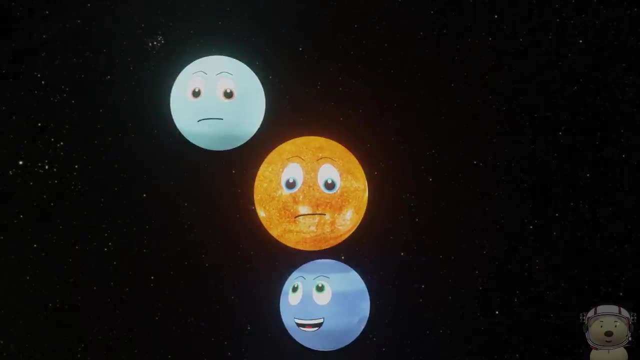 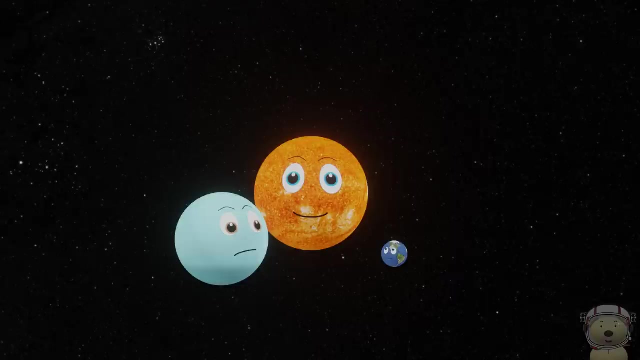 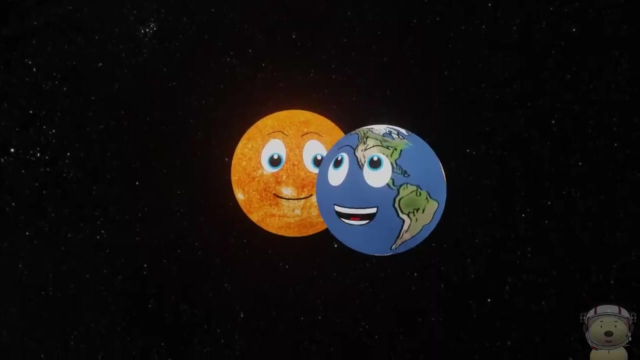 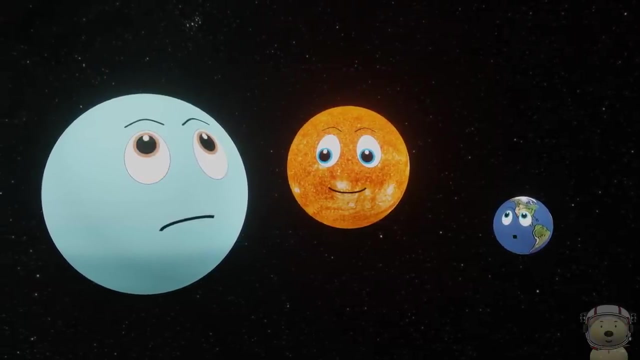 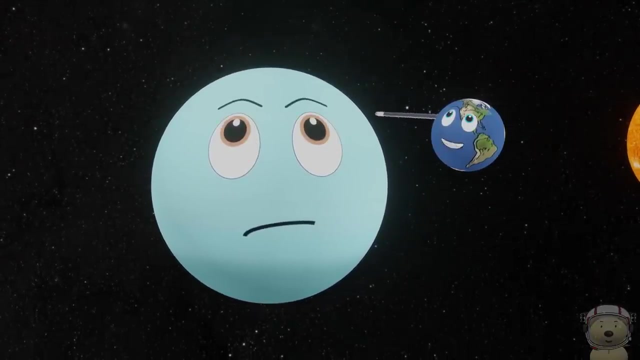 Never to be seen again. Whoa, Whoa, Uranus- Really Whoops. Second ingredient: Gravity. I don't see anything Brilliant. Thanks, Uranus, That has really improved the video. Accuracy is important. Let me erase your bit of gravity then. 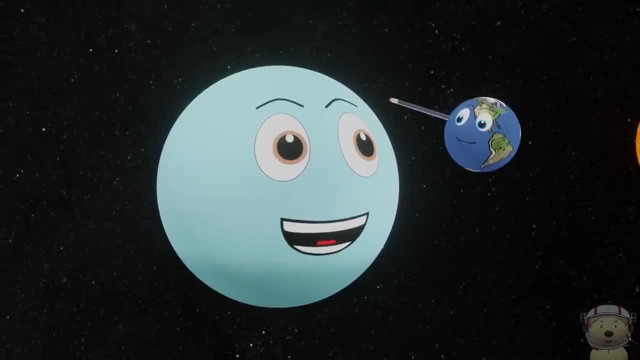 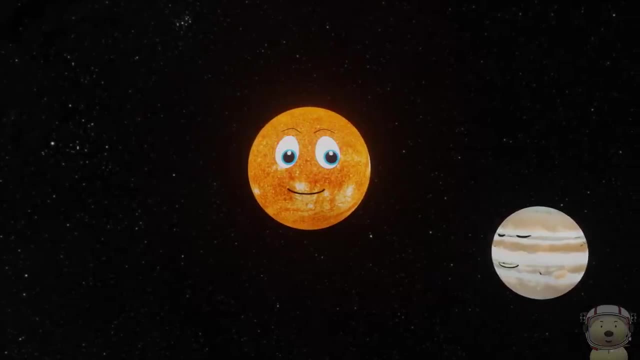 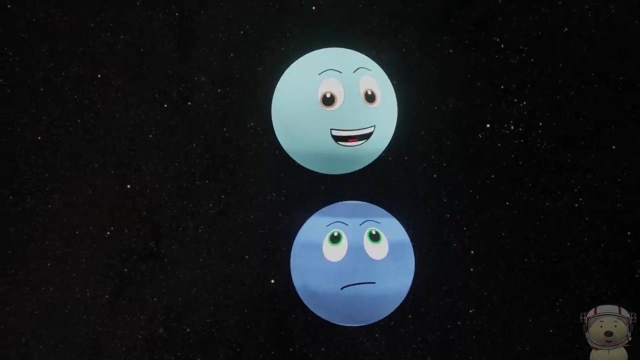 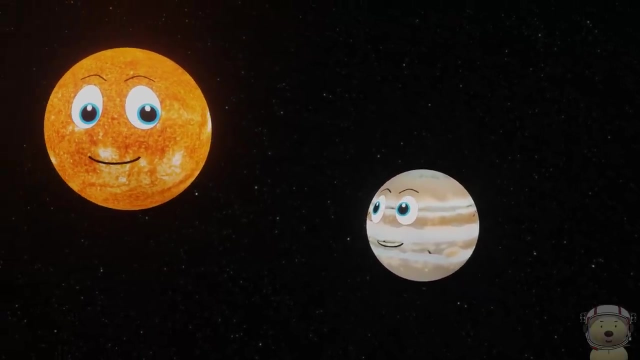 Ha, That is never going to work, Hahaha. The third ingredient: Planets. Watch it, Hey, Not that I was here first. Guys, guys, Not just any old order. We have an order. Play the Toy Time Town Planet Order ditty please. 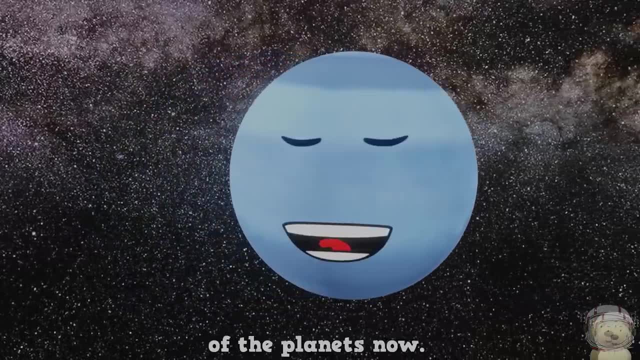 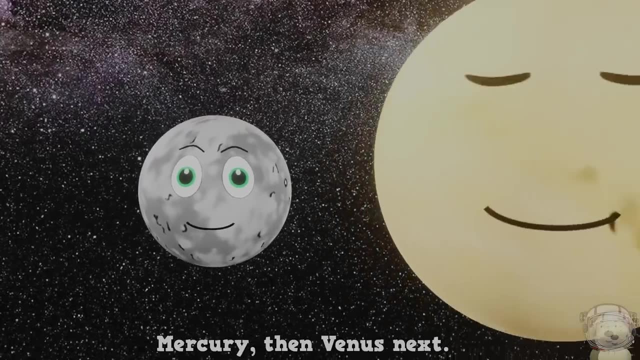 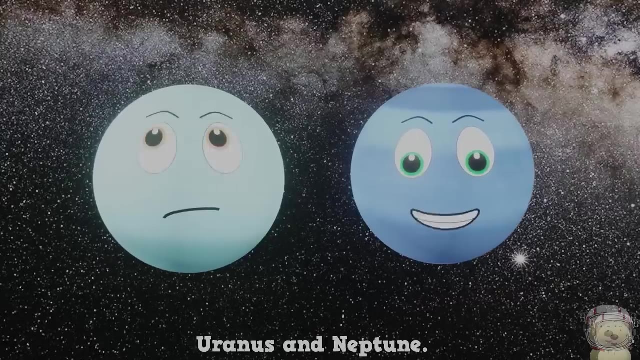 It's time to learn the order of the planets. now Planet order is: Mercury then Venus, next planet Earth, then Mars- who's red Big Jupiter, then Saturn, too Uranus and Neptune. Mercury then Venus, next planet. 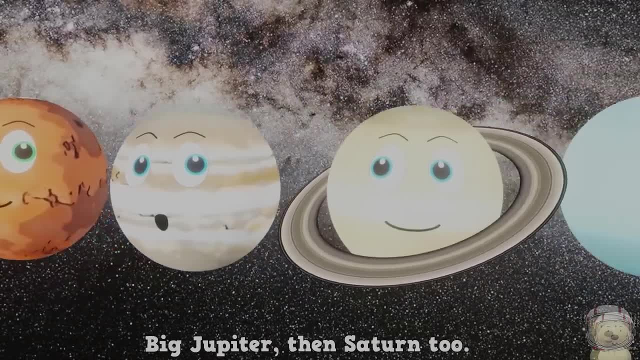 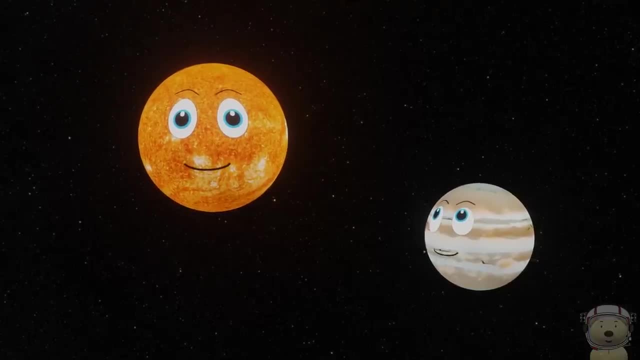 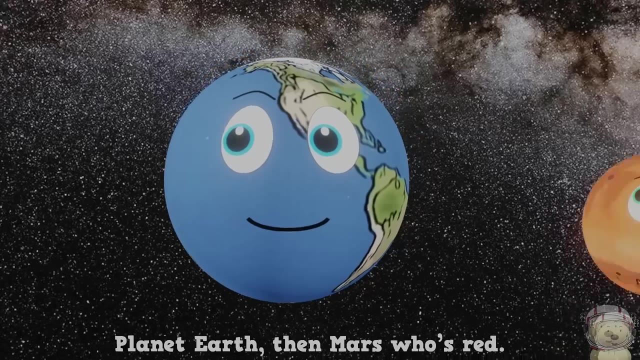 Earth, then Mars. who's red? Big Jupiter, then Saturn too, Uranus and Neptune- Better, First we need the rocky planets: Neptune, Mercury, then Venus, next planet Earth, then Mars. who's red? 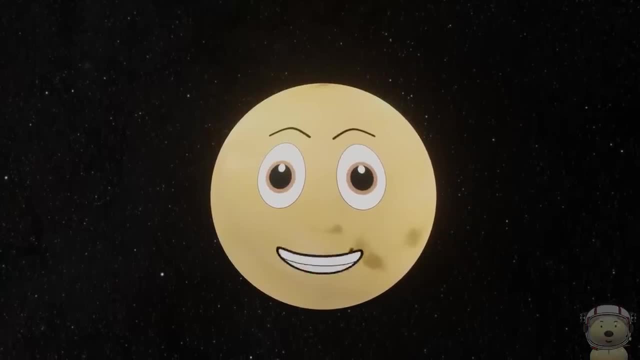 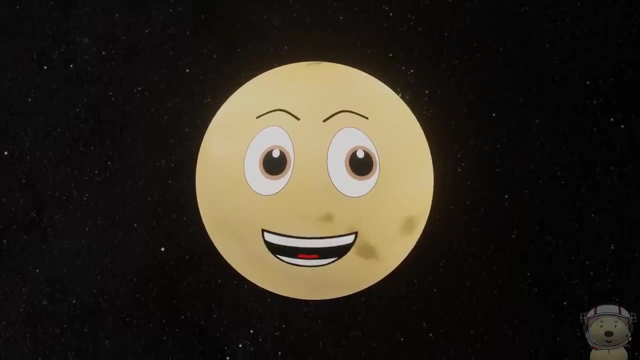 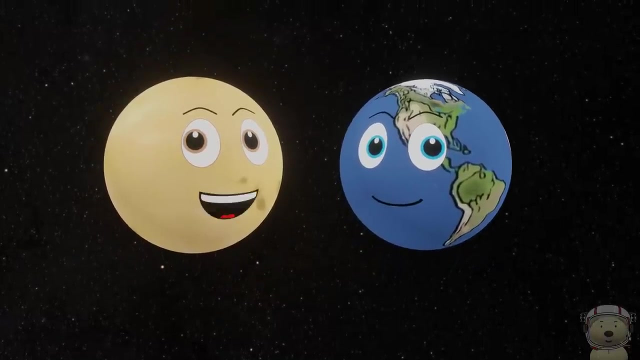 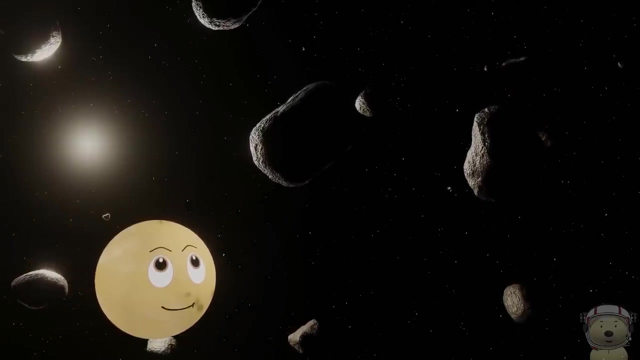 That's the first bit of our solar system. Pretty cool, eh? Next, before the gas giants. What do we need, Sweets? No, we need asteroids and meteoroids, And lots of them. An asteroid is a small rocky body orbiting the Sun. 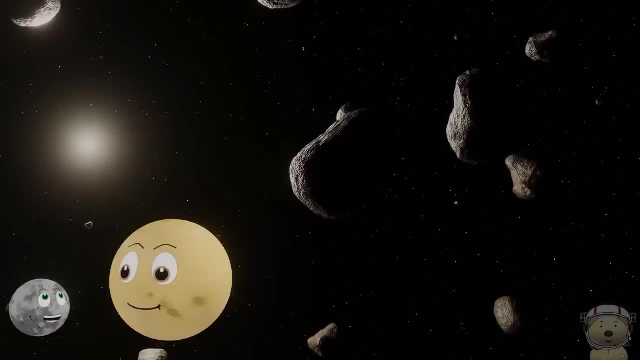 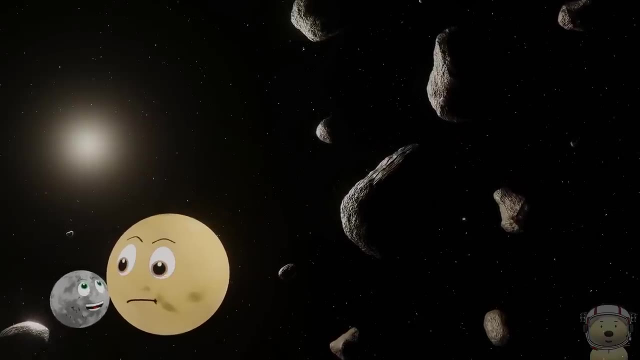 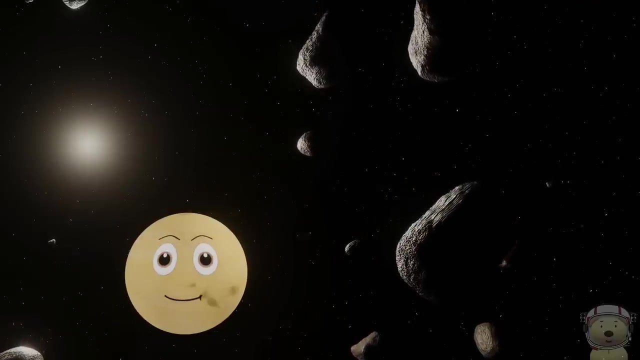 What? These guys have hit my surface in the past and caused loads of craters. Let me at them. Let me at them. No, leave them, Merc. They're not worth it. That's the asteroid belt between Mars and Jupiter sorted. 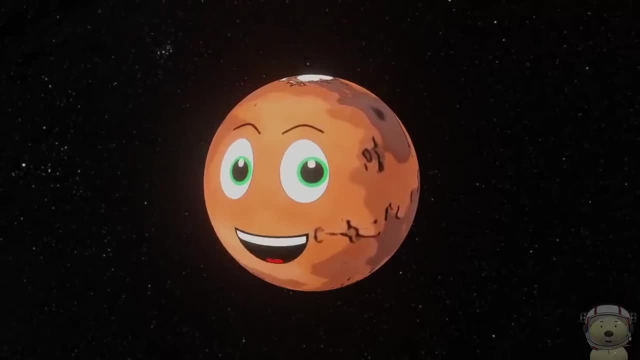 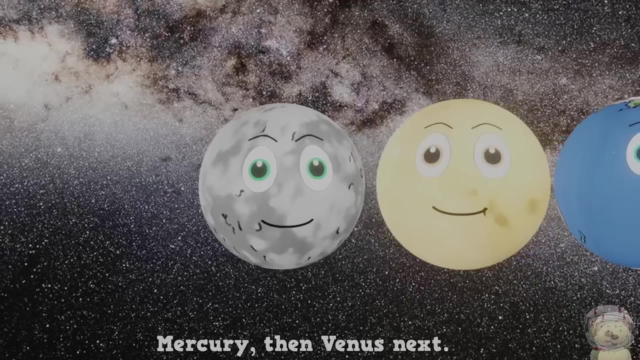 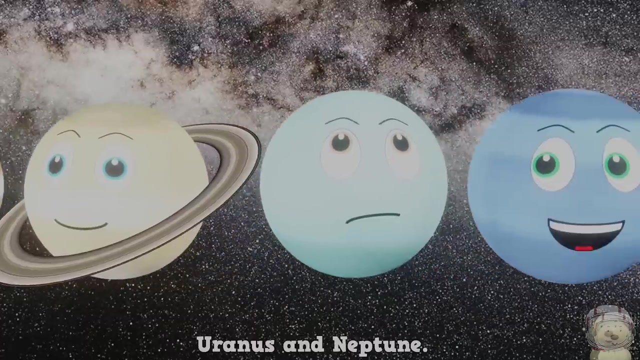 Next up the gas giants: Neptune, Big Jupiter, then Saturn, too Uranus and Neptune. Mercury then Venus, next planet Earth, then Mars- who's red? Big Jupiter, then Saturn, too Uranus and Neptune. 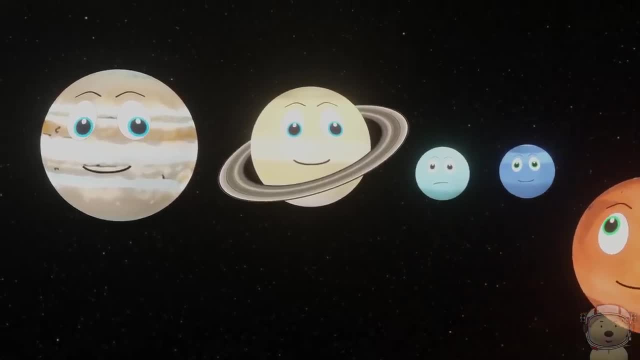 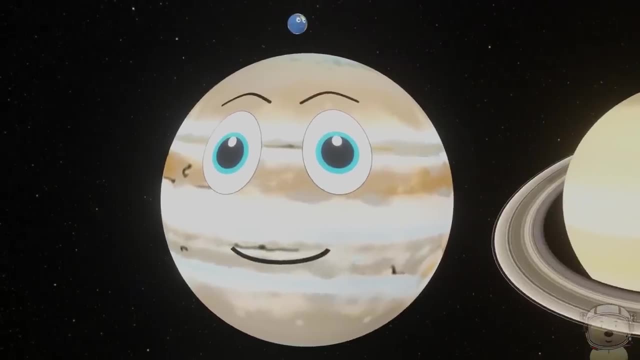 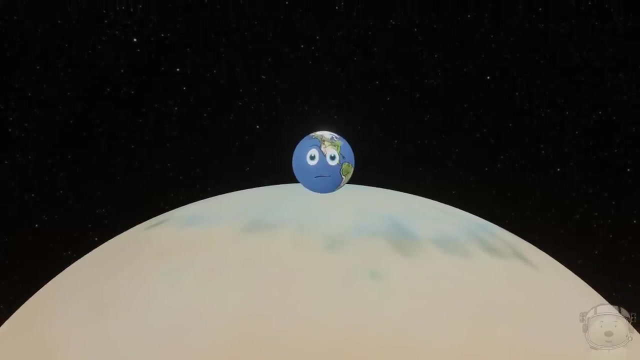 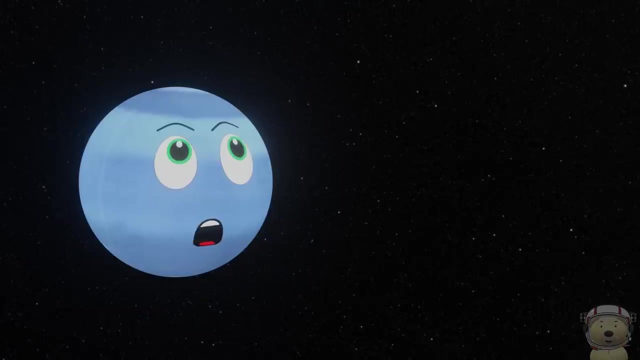 They are much bigger than the rocky planets. They are balls of hydrogen and helium. You couldn't stand on the surface of these planets because they are not solid. Wait what Uh-oh Next ingredient up more asteroids and comets. 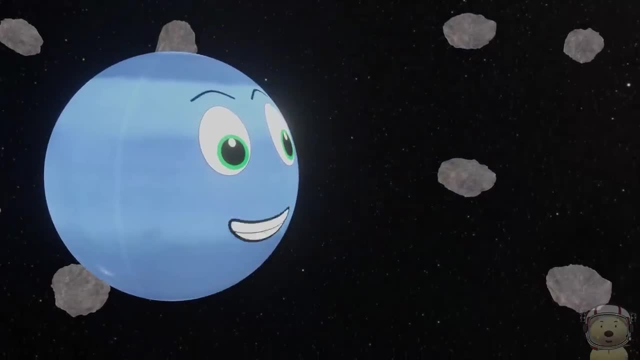 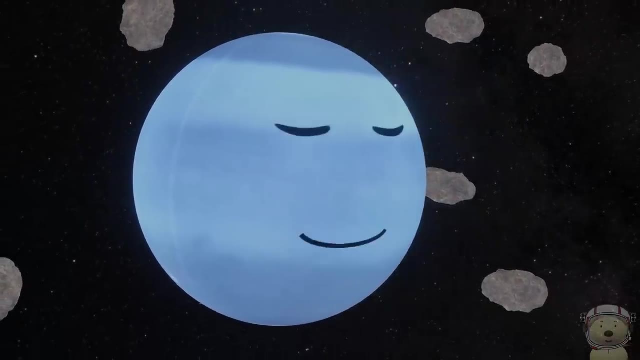 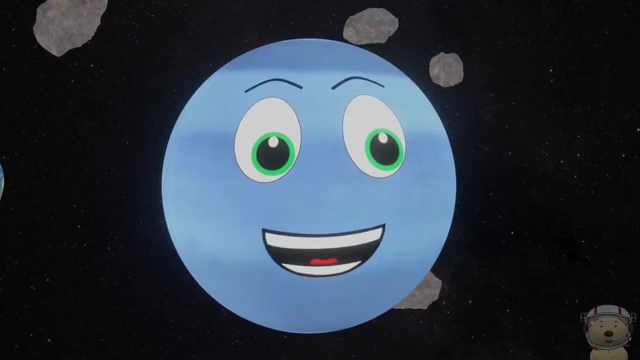 Beyond me lies a region of space filled with icy bodies, known as the Kuiper Belt. This holds trillions of icy objects. Hey, Neptune, I've got a cold joke for you. Uh, Sorry, Earth, I have some place to be. 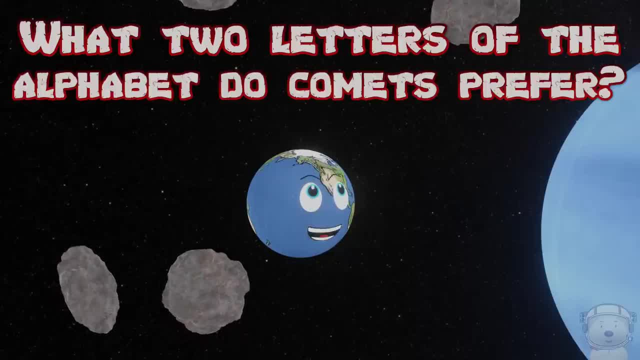 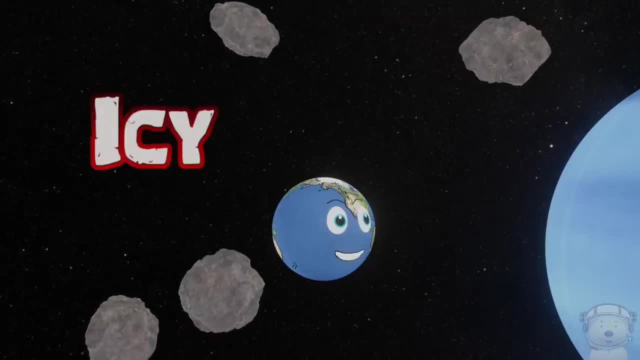 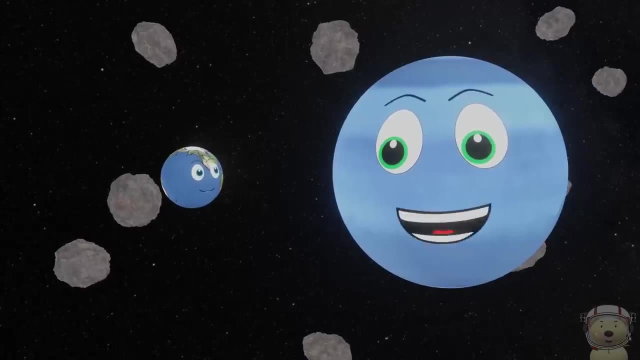 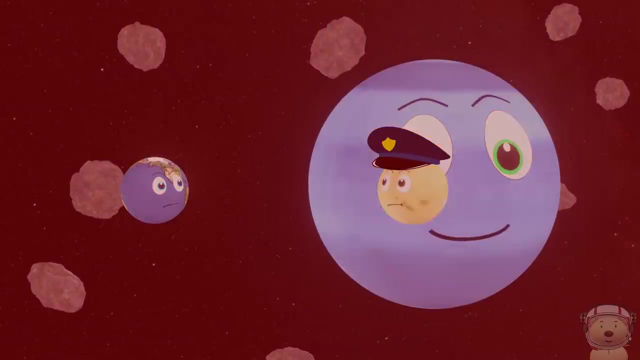 What two letters of the alphabet do comets prefer? Uh, I don't know. I see Icy. I see Icy. I see somebody that needs to be removed: Venus stickle. Come with me please, sir. 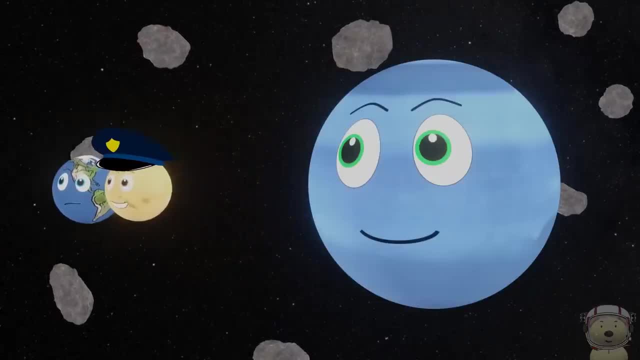 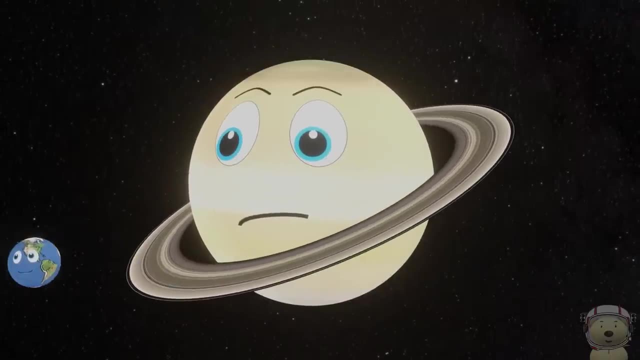 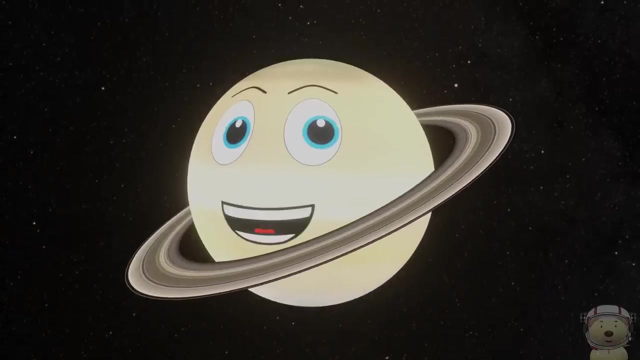 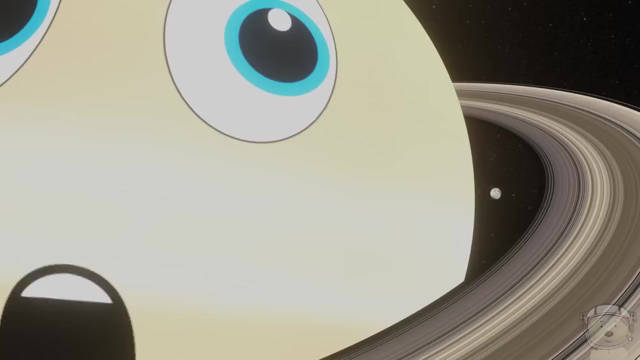 But I For that cold joke. you are under a vest. Next up, dude. Make way, Mirk, we got a runner, Let me at him. Uh, Next up, dudes. we need another ingredient: a sprinkling of moons. 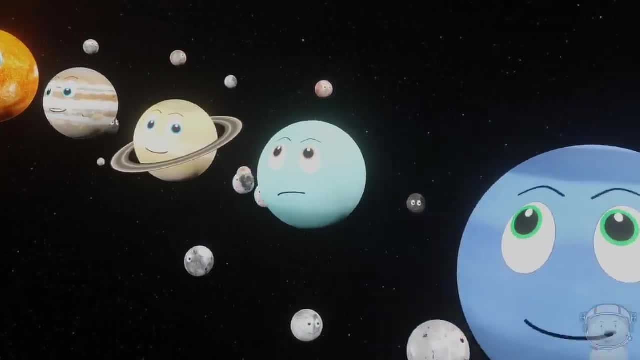 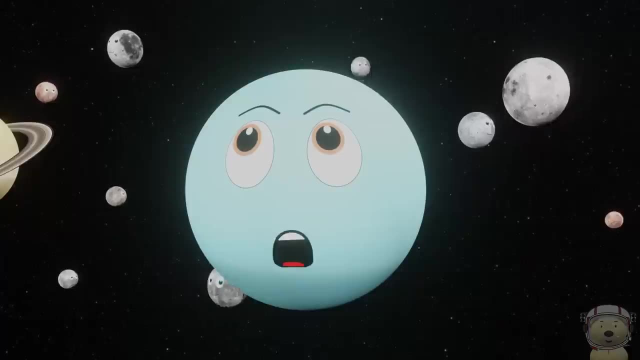 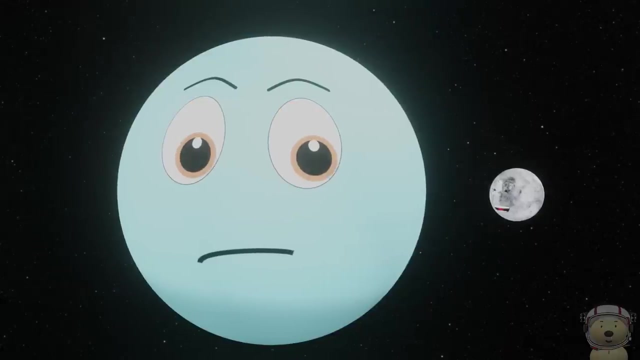 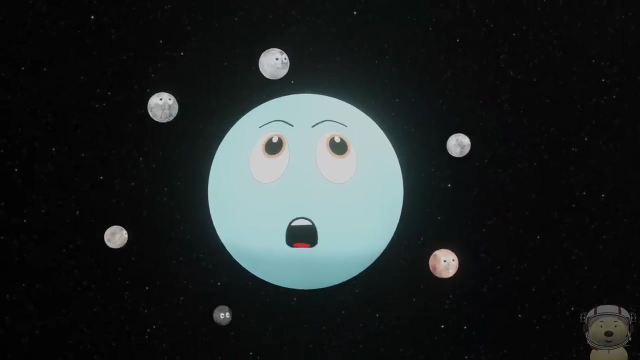 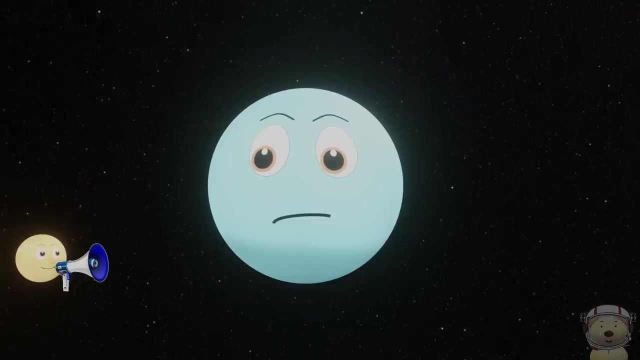 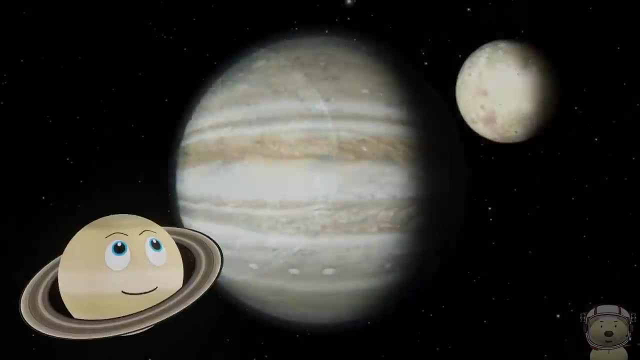 Wait, wait, quieten down you lot. No, no, stop that, stop that. I will not tolerate unruly moons. What? No, stop that. Don't have fun. Moons quiet please. No problem, Now Earth only has one moon, But there are more than 200 moons in our solar system. Most